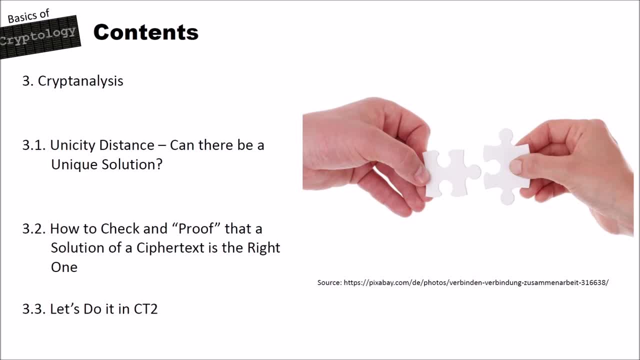 prove by yourself if a solution you just found is the correct one, or maybe it's not. And finally, we want to have a look at how to do it in Crypto2.. That means that we will have a look at the Unicity Distance of the Mono-Alphabetic Substitution cipher in Crypto2. 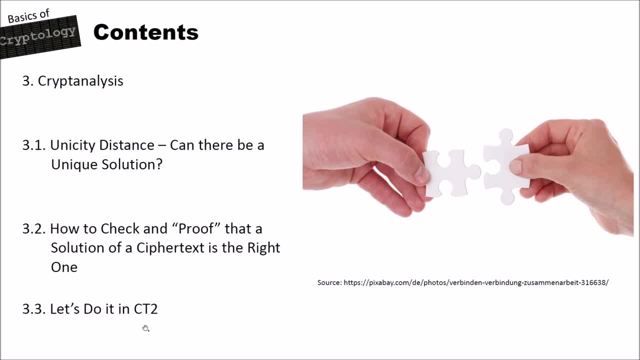 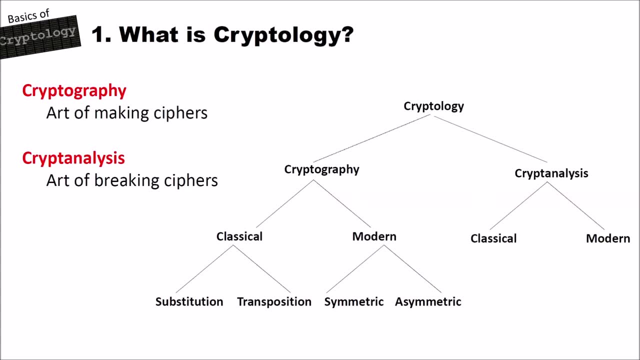 and we want to have a look how to solve the Zodiac Killer Z408 message and how to convince us that the solution we found is the right one. As with all this, let's get started In the videos in this series. here I first have a look at this graph here And, as we all know, 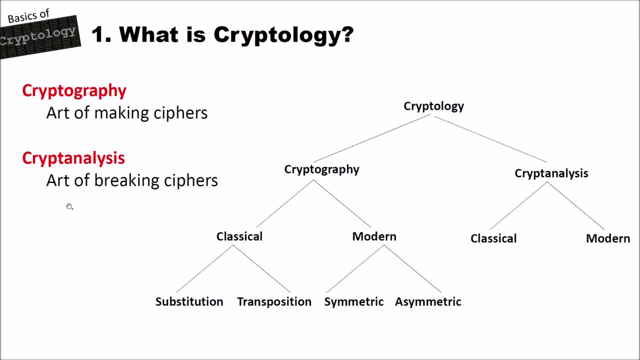 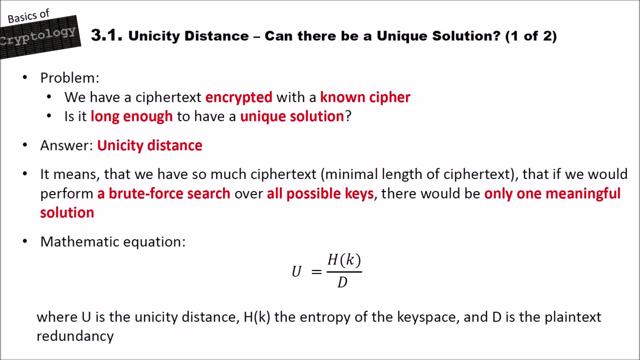 cryptography is the art of making ciphers and cryptanalysis is the art of breaking ciphers, And in this video we want to have a look at cryptology, cryptanalysis, classical and modern cryptanalysis. Let's speak about Unicity, Distance and the question: can there be a unique solution? 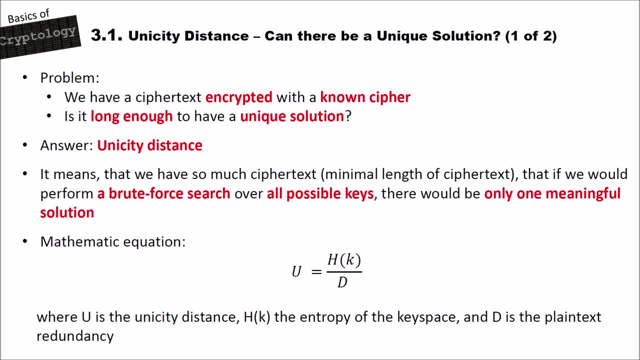 to a given ciphertext And the problem is that we have a ciphertext encrypted with a known cipher, So we know the used system that was used or the globe that was used to encrypt plain text to get ciphertext. So the question is: is the ciphertext long enough to have a unique solution? 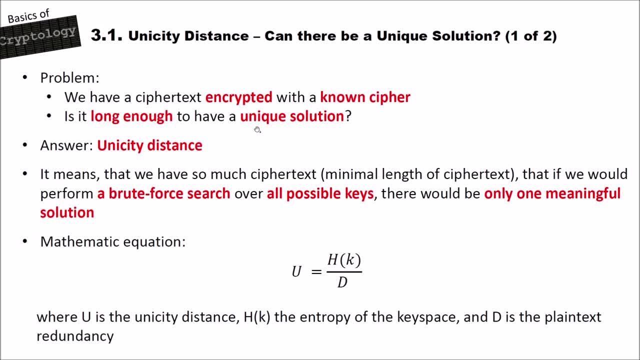 So can we find the solution with a unique key Or is there a key giving us a unique solution? Is the ciphertext long enough to have a unique solution, Or is there a key giving us a unique solution? And the answer to that question is Unicity, Distance. 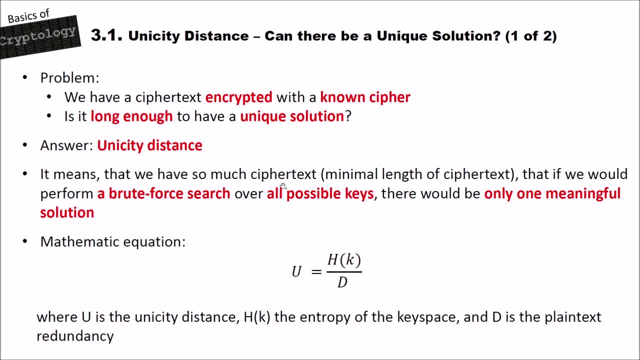 Unicity Distance means that we have so much ciphertext of a given a given blocks tube- that is as long as any type of anchtenode cipher or used to encrypt of a given cipher- that if we would perform a brute force search over all possible keys of the used cipher, there would be only one meaningful solution. 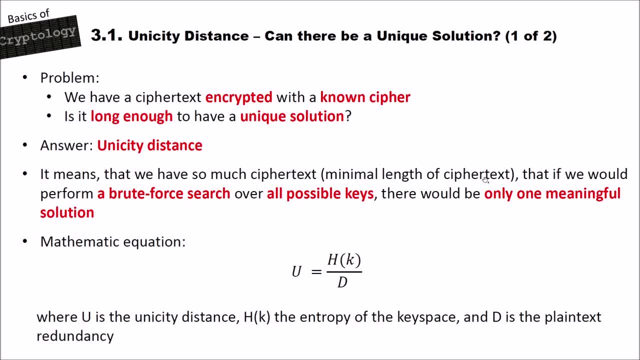 And so much ciphertext is a minimal length of ciphertext. And for this unicity distance, that is that here exactly we have a mathematic equation And that is: u equals to h of k divided by d, where u is the unicity distance, h of k the entropy of the key space. actually, 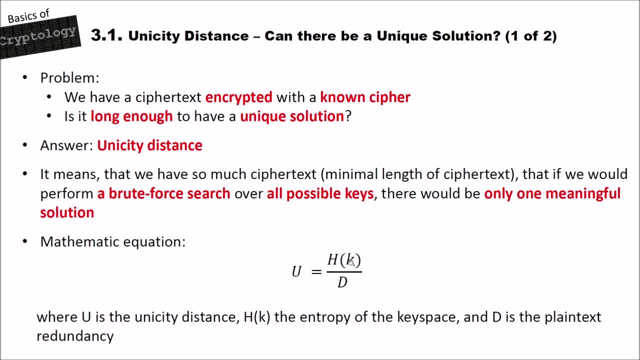 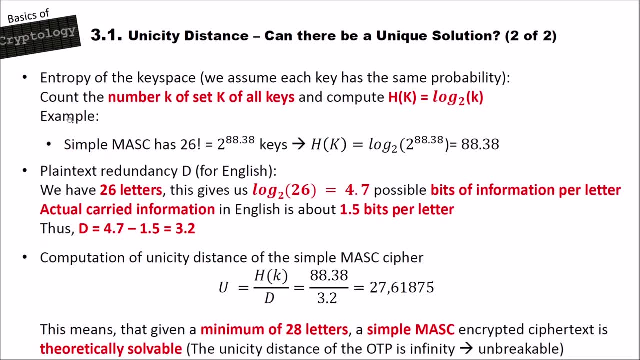 this case here is to be uppercase. This is not lowercase, as you will see on the next slide. And d is a plaintext redundancy here. First of all, the entropy of the key space in our equation, And we assume each key has the same probability. 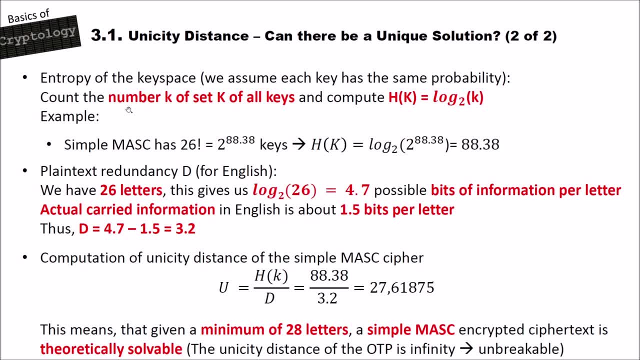 And the entropy of the key space can be computed by counting the numbers. lowercase k here, or byorro部. you can do that by, or. we would also use the uppercase D as well as d of the set of uppercase K. this is the key space. 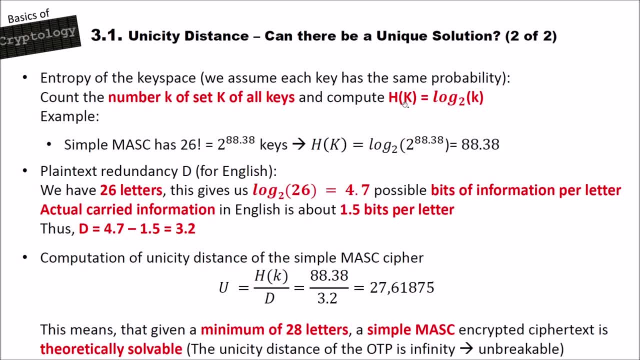 of all keys and compute the entropy by taking the logarithm of base two to the number of all keys. And here's an example for the simple mono-alphabetic substitution cipher. And by the way, I of course only show you this here. 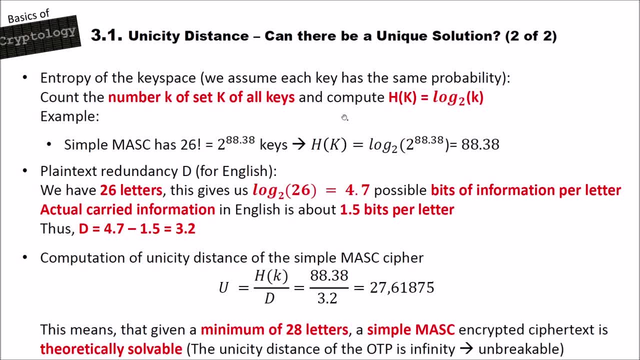 I will not show you the proof that this works, but believe me, this really works. And the simple mono-alphabetic substitution cipher has 26 factorial keys. This is about two to the power of 88.38 keys And with our equation here follows: 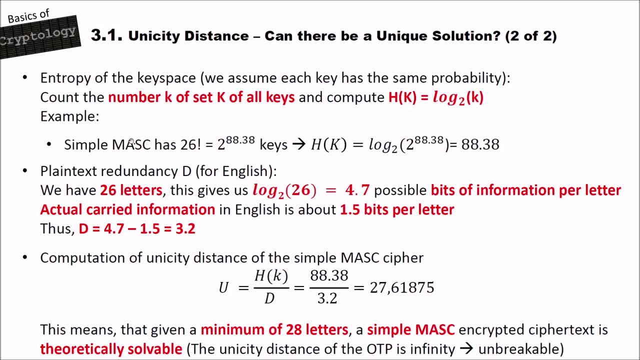 that the entropy of this key space of the mono-alphabetic or the simple mono-alphabetic substitution cipher is the logarithm of base two to this number, So we can just eliminate this two here- And the entropy of the key space of the simple mono-alphabetic substitution cipher is 88.38.. 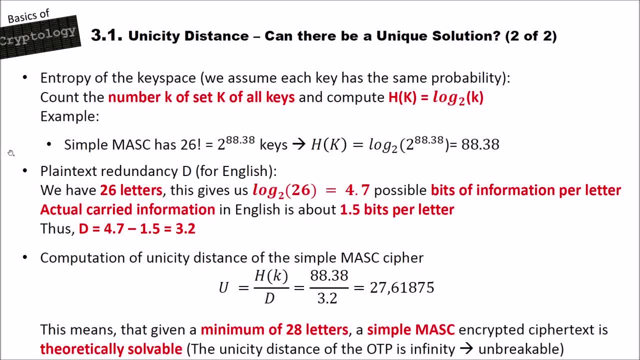 Now let's speak about plaintext, redundancy D, which we also need to compute this unicity distance for the English language. With the English language, we have 26 different letters and this gives us 26,, or the logarithm of base two of 26,. 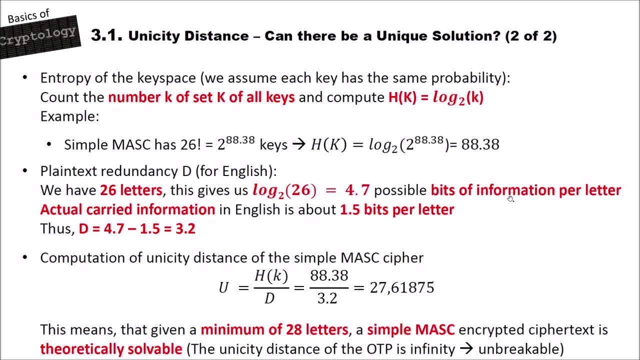 which is equal to 4.7 possible bits of information per letter for the English language But languages highly redundant. That means that the actual carried information in English is only about 1.5 bits per letter, So you could store the same information in English sentences Instead of. 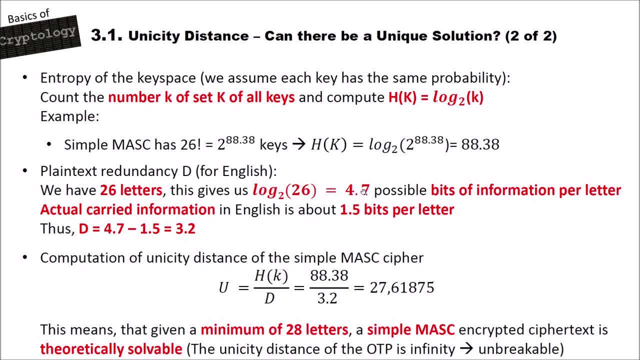 using 4.7 bits to store the information. you can only use 1.5 bits to store this information and you would not lose any information. How do we get these 1.5 bits per letter? That's a good question. 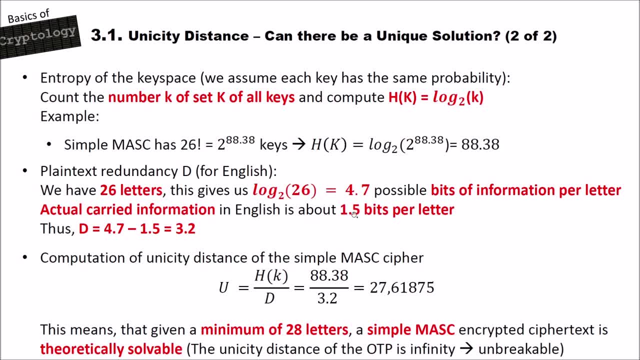 You, for instance, take English text and then, when you compress these texts using, for instance, compression algorithms, you will see that, instead of needing these 4.7 bits for these texts, you only need 1.5 bits. So this is a minimal size needed for compressing this English. 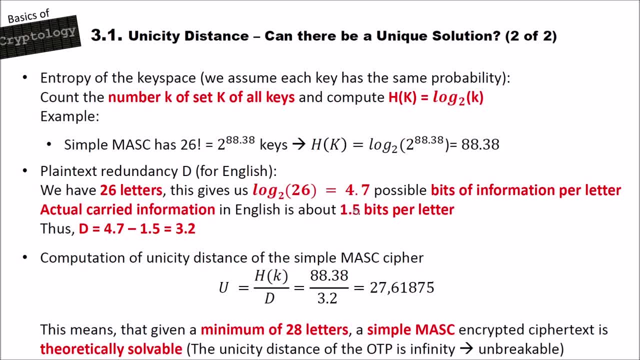 information And this is the information that is actually carried per letter with English. So to calculate the redundancy of the language we take these first 4.7 bit information here, we subtract the actual carried information- 1.5 bit here, and we got 3.2. And now we can compute the unicity. 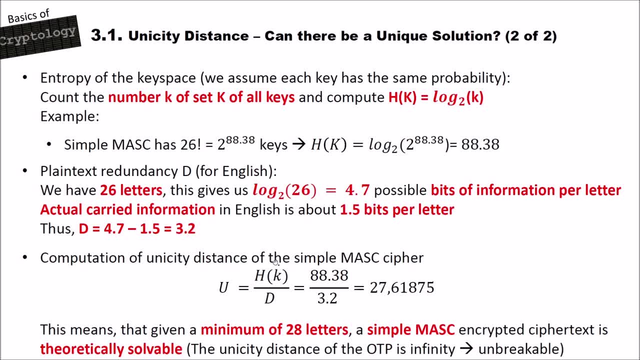 distance of the simple mono-alphabetic substitution cipher easily by just taking the entropy of the key space here, this H of k- this also has to be an uppercase K divided by the redundancy d and we just enter our numbers here. So we have 88.38 entropy of the key space. And if 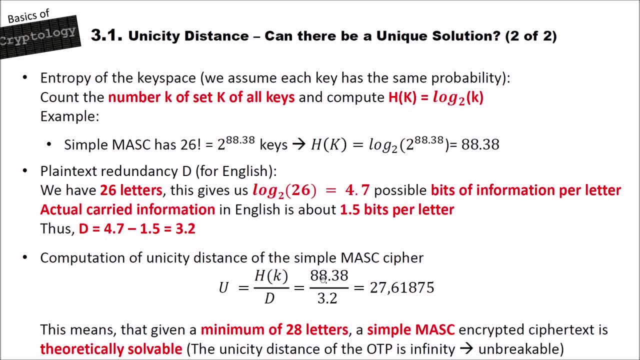 you don't know what entropy means. I also made a video about entropy in cryptography and you can have a look at this video. It's also part of the series And we divide this 88.38 by our redundancy 3.2.. 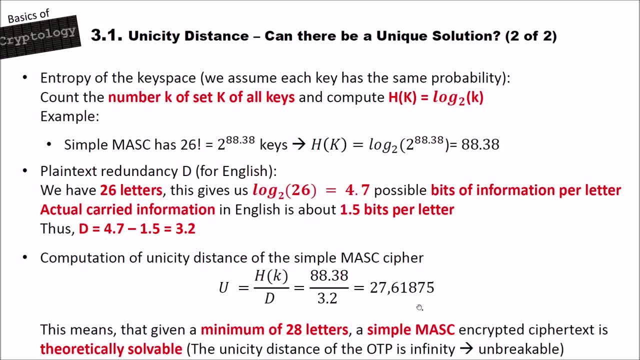 get this 27.61875.. So we have 28 letters as a unicity distance. That means that, given a minimum of 28 letters, a simple monalphabetic substitution and ciphered, encrypted ciphertext is in theory solvable. And if we have less letters then we probably have not only one solution, we have more. 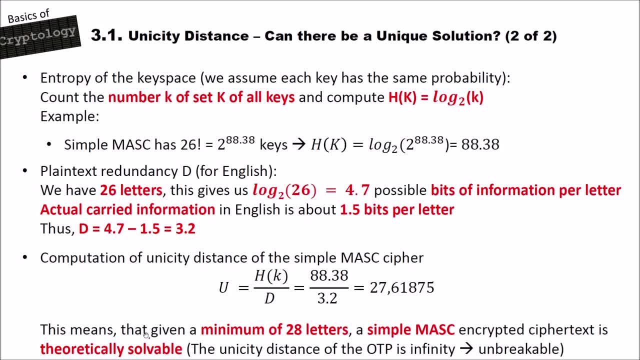 solutions. That means we can find different keys for shorter ciphertexts than 28 letters. that give us two valid texts And we cannot distinguish as an attacker which of these two texts is the right one. What that means we will see later in Crypto2 when I try to break. 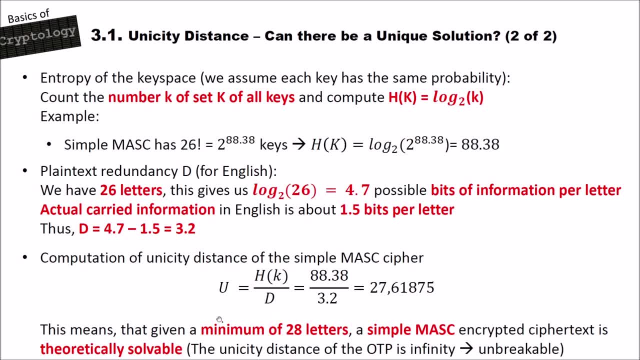 very short ciphertexts that are actually below the unicity distance of the simple monalphabetic substitution cipher And, just as a fact, the unicity distance of the one-time pad. this is the one perfect cipher that we know. I also made a video about this in the series. 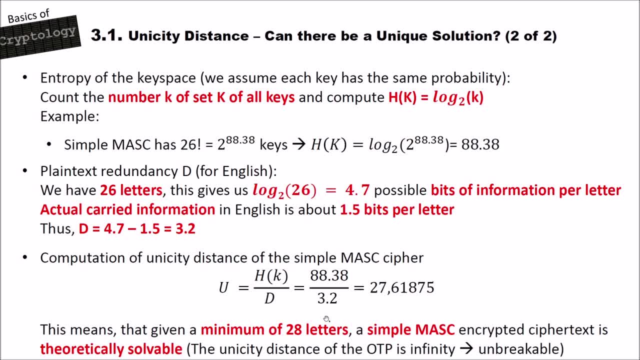 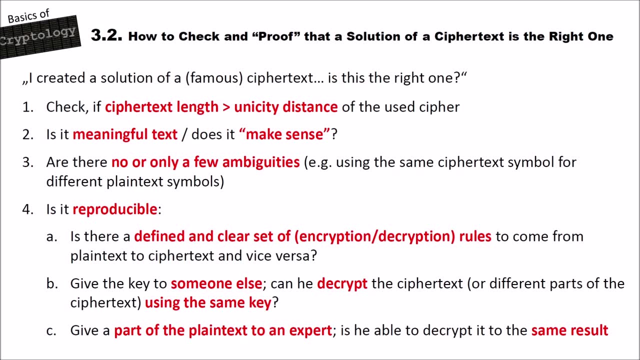 is infinity. That means that the one-time pad is really unbreakable, And the unicity distance also tells us this. So we would need infinity letters to break the one-time pad, which is, of course, not possible. Now let's talk about how to check and prove that. a solution of a ciphertext. 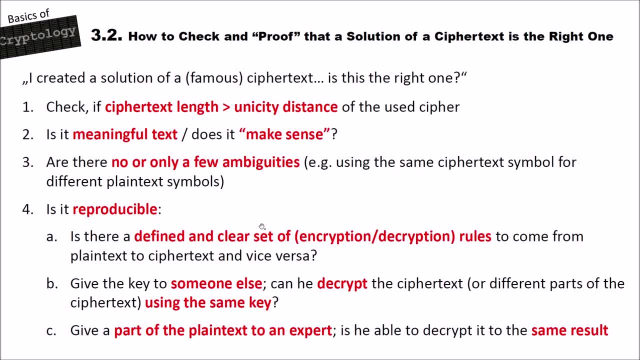 is the right one And, as I said in the beginning of this video, there are some people that, if you reach me and tell me I created a solution of a famous ciphertext, I broke this. I broke the Voynich manuscript, I broke Cryptos K4, I broke and you can enter any unknown famous 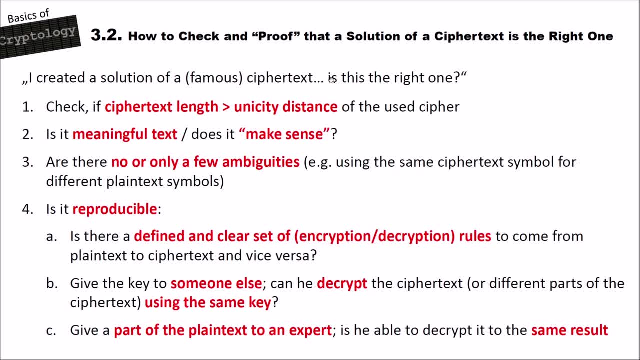 or not so famous cipher here And they want to know: is this the right one, Or how can they prove that this is the right one? And I sat down and thought of how can we deal with this problem And how can people check this, And how would I check if a solution is the correct one? 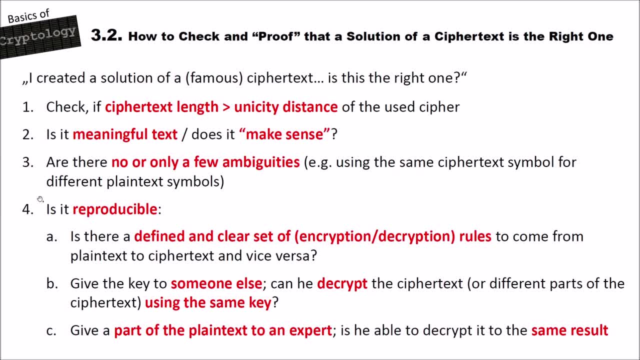 And I made this list here with four points and this four point here with some sub points, Of course, when you have a solution of a ciphertext, first check if the ciphertext length is greater than the unicity distance of the used cipher, For instance. there are some people on. 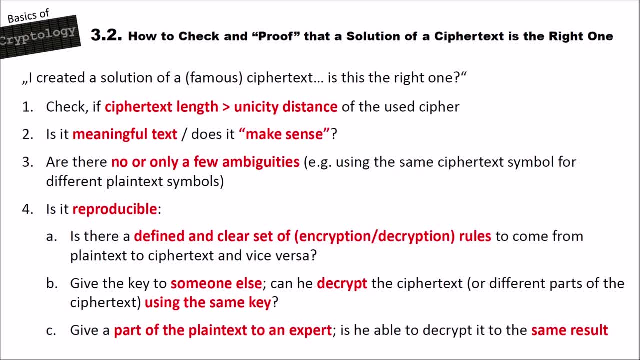 Facebook that post ciphers of mono-alphabetic substitution ciphers of length five, So only five letters. And then they ask: please solve this. But actually this is not solvable. You can find many solutions for a five letter ciphertext And since that you should first check if my ciphertext 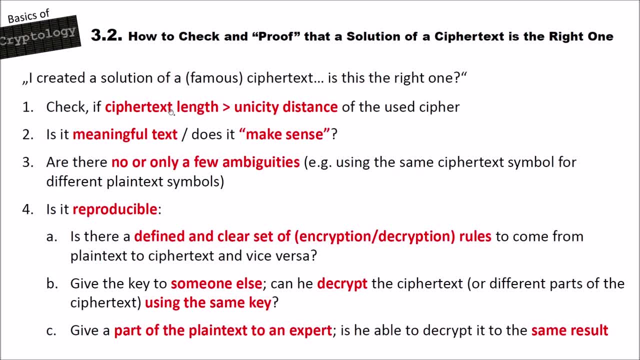 if you want to create a challenge, for instance, has a length greater than the unicity distance. That doesn't mean that there are no ciphertexts longer than the unicity distance that also have different solutions. This can also happen, But below the unicity distance. 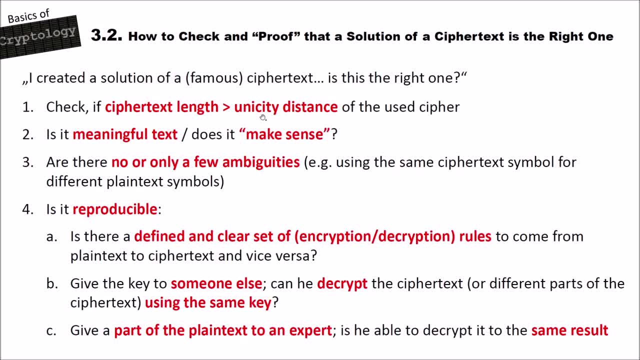 we are quite sure that there are probably a lot of more solutions to the ciphertext. The second point on my list here is: is it meaningful text or does it make sense? So you decrypted a ciphertext, You have now the plaintext and you can read it. And does it make? 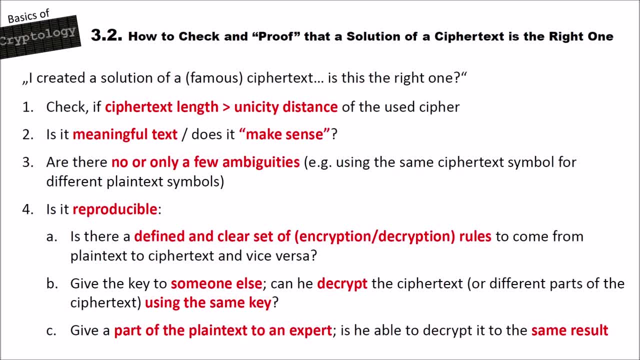 sense. For instance, when you decrypted a ciphertext from a noble man from the 16th century and he's in your plaintext, you have something like modern machines, science fiction and so on. This is not meaningful. That would not be part of a ciphertext. 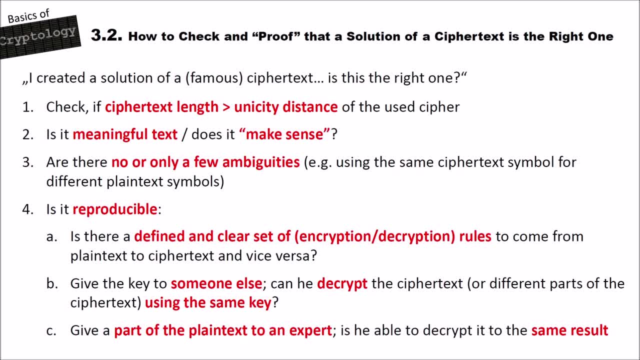 Or a plaintext of the 16th century, And you can look at the environment where this text has been created. Does it make sense in that area? And also, is the text inside meaningful text Or are there a lot of errors? Or can you read all the words correctly? And with that we come to the third part on 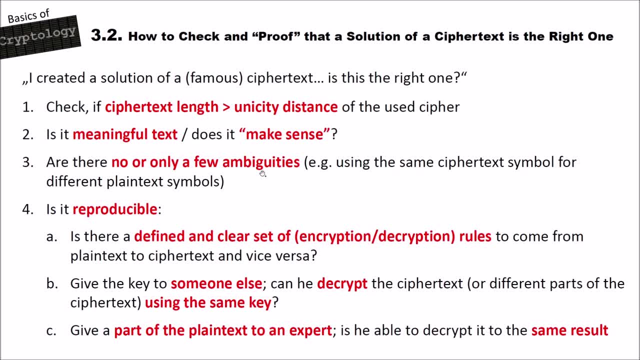 my list Are there no or only a few ambiguities. That means that, for instance, the same ciphertext symbol was used for different plaintext symbols. So there are really people that give us solutions to ciphertext And then on one place they use the ciphertext letter X and they decrypt it with an A. 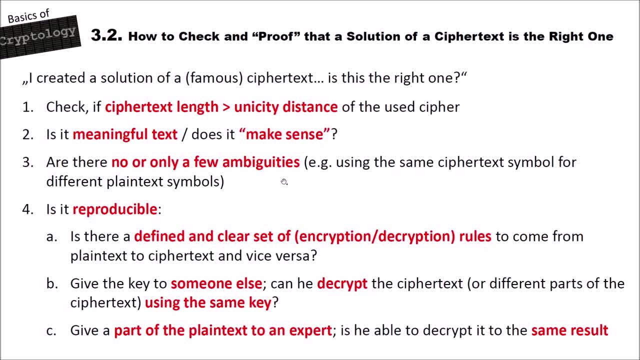 but that doesn't fit in another position. So they decrypt this with a B or with a C, And when you have a lot of these ambiguities, you can be 100% sure that this is not the correct solution. Sometimes you have these ambiguities, especially when you have. 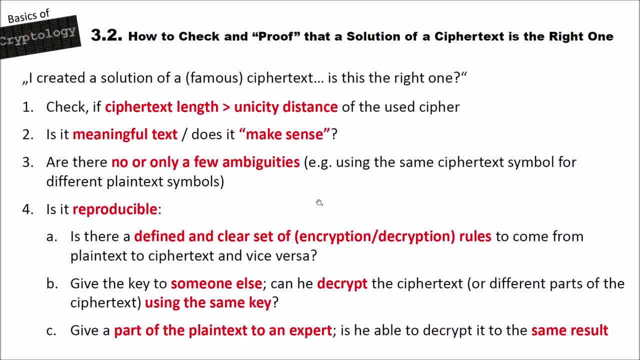 a lot of ciphertext with errors. So when you have original encrypted manuscripts from the 15th, 16th, 17th century, you have probably a lot of errors. Also with original Enigma messages that were captured. these were sent using Morse code and the receiver or the eavesdropper that 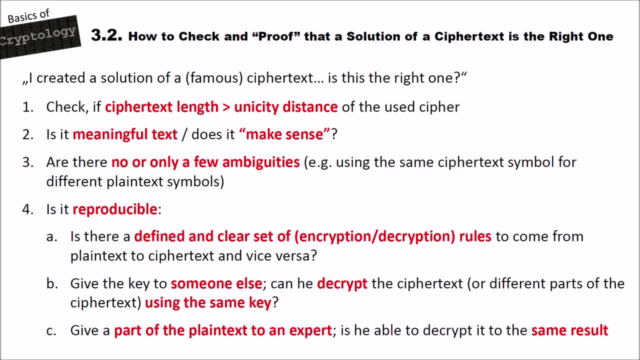 received the message also and wrote it down, probably made some errors, So you can have errors in your message, But if most of the letters are erroneous, can also be sure that this solution is wrong. and now i come to the fourth and i think most important. 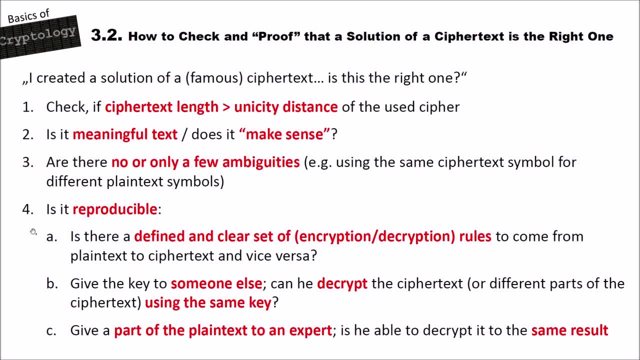 point on my list here, and that is: is your solution reproducible? that means a. is there a defined and clear set of encryption, decryption rules to come from plaintext to ciphertext and vice versa, and also, are these not too complex, not too complicated? of course, you can find 100 rules from one ciphertext. 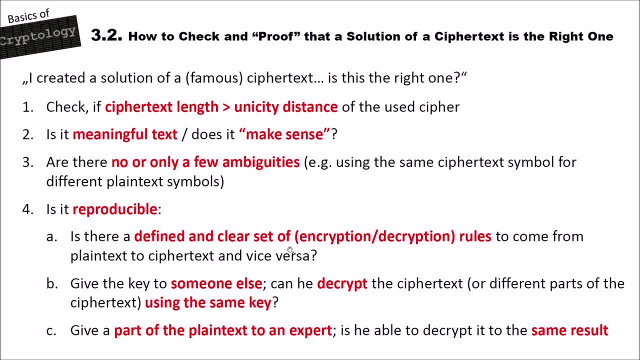 to a solution, to a plaintext, and when you follow these 100 rules then you get valid plaintext. but in fact that means that you can create with these 100 rules probably all solutions that you want to create. so these rules should be easy, so that the original sender of the message or the 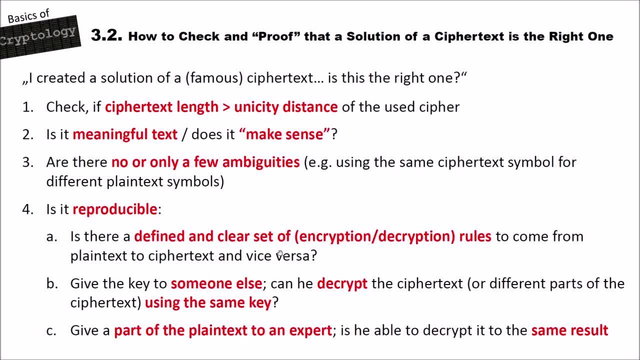 creator of the message could actually follow these. point b on my list here is: give the key to someone else and then check: can he decrypt the ciphertext or different parts of the ciphertext using the same key? for instance, you have a ciphertext of one page and you decrypted half. 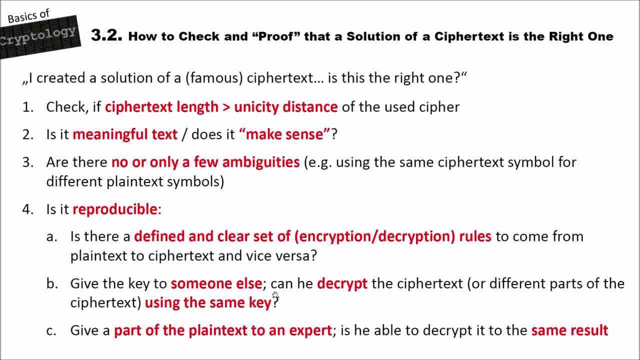 of the page. then you give the ciphertext- the second part, which is encrypted using the same key- to a different person. you give the key to that person and you decrypt the second part, which is encrypted using the same key, to a different person. can he or she then decrypt the second part of the ciphertext, or maybe also the complete ciphertext? 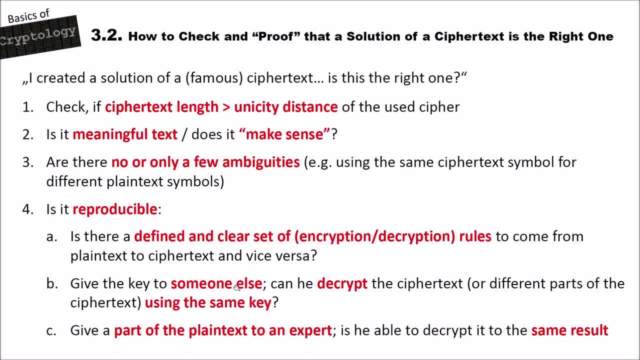 using your key. if he can do this and all the other points on my list here also are true, then probably you have the correct solution. and finally- and that was done, for instance, with the Zodiac Killer case- gives a part of the plaintext to an expert and if he or she is able to decrypt it, to the same result. 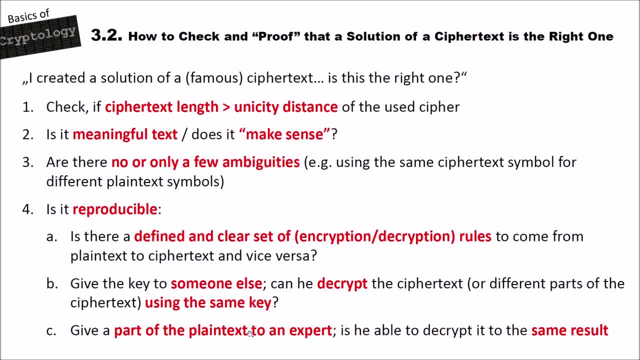 that probably is also the correct solution. if the Zodiac Killers message that 408, that was done that way. so you had this Donald and Betty Hahn that were just normal people that decrypted the original Z 408 message of the Zodiac Killer and they gave it to the police and the police gave their solution. but 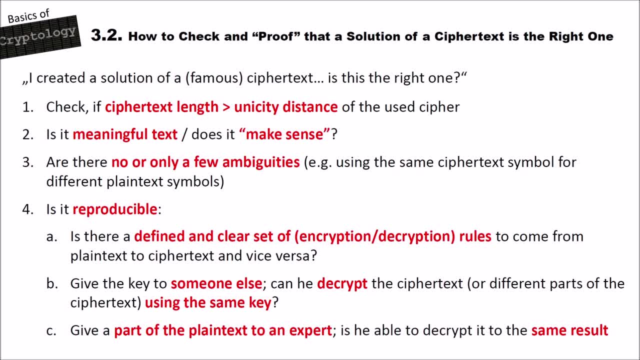 not the complete solution, only a short part, the first sentence, to a crypto expert. and the crypto expert was also able, based on their solutions and of course, using his knowledge, to come to the same solution. so he decrypted the text to the same plain text. so they were sure that the solution of the Hardens 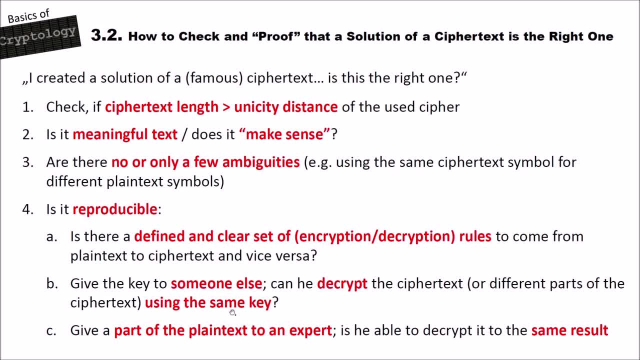 were, or was, the correct solution, and you could do the same. just decrypt only a part, or only give only a small part of the plain text to an expert, like the first sentence, and if he or she is able then to decrypt the rest, then your solution is probably the right one. 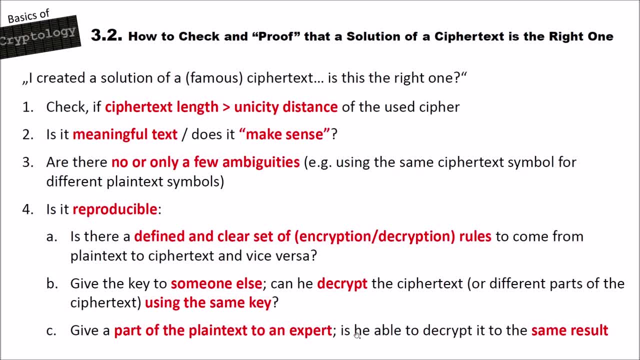 as an example. for instance, if you would have solved the Voynich manuscript and you have the key to decrypt it, then give it to an expert and ask him: please decrypt just another page. of course, under the assumption that the Voynich manuscript was encrypted using the same key on all pages to 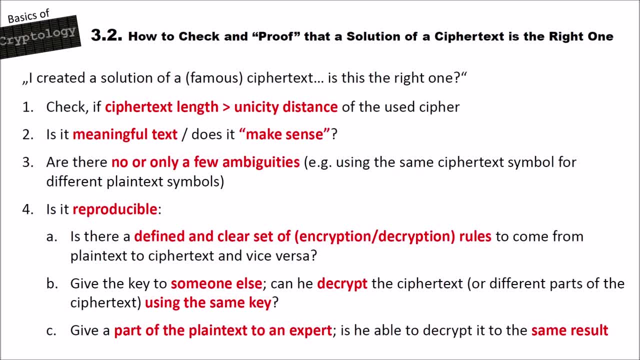 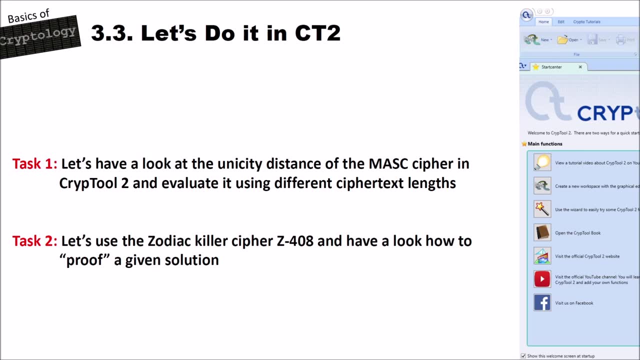 decrypt it and if he or she then is able to decrypt another page using your keys, and probably you have solved it. if one of these points here does not apply to your solution, then probably your solution is a wrong one. now let's do it in crypto 2.. I have two tasks. 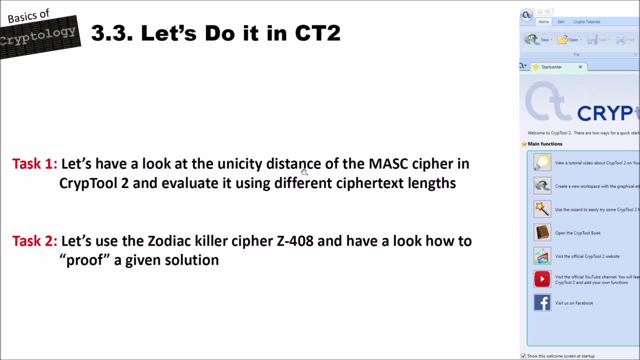 the first task is: I want to have a look at the unicity distance of the simple mono-alphabetic substitution cipher in crypto 2 and I want to evaluate the unicity distance, or at least have a look at the unicity distance, and to make clear what it means using different cipher text lengths. 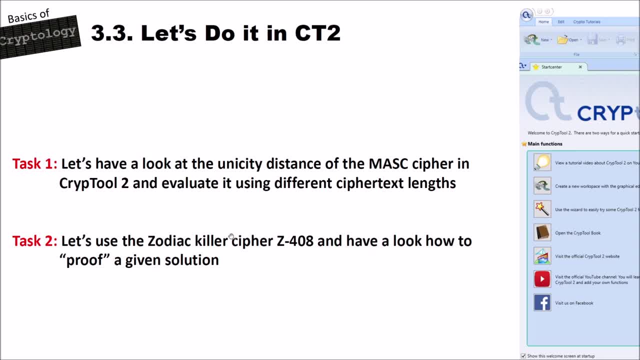 and then I want to have a look at the Zodiac killer, cipher z408. this in crypto 2 and I also made a video about this, but I want to show you how to solve it, let's say by hand, and how only a part can help an expert to solve it actually, and how we then can prove the. 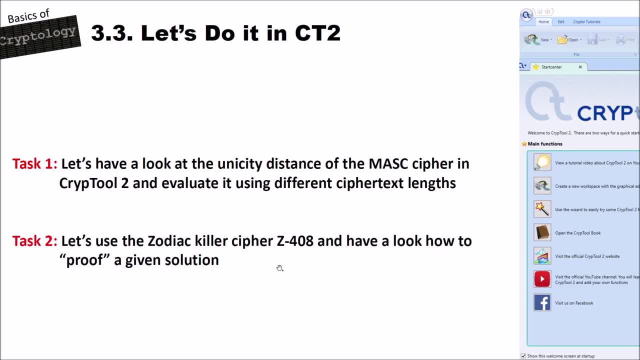 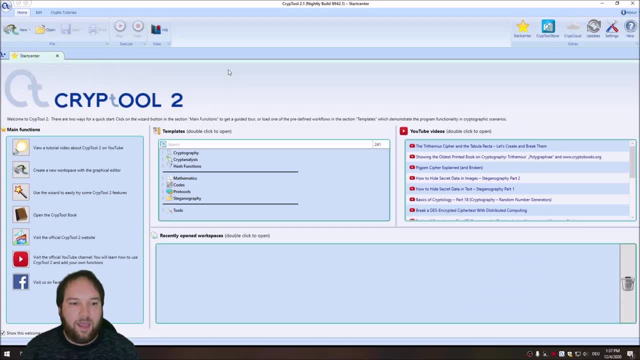 given solution, for instance in crypto 2 with the mono-alpha homophonic substitution analyzer. I'm here now in crypto 2 at the start Center, and I want to evaluate the unicity distance of the simple mono-alphabetic substitution cipher. to do so, we first have to create a nice 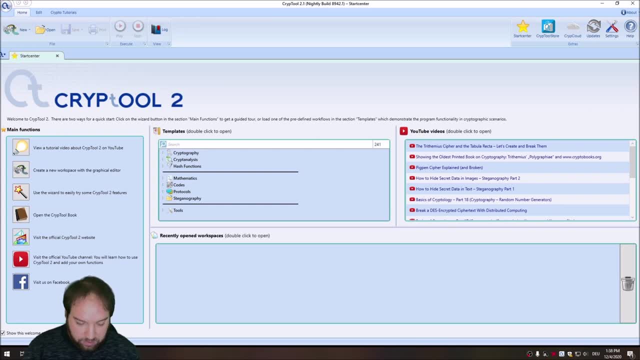 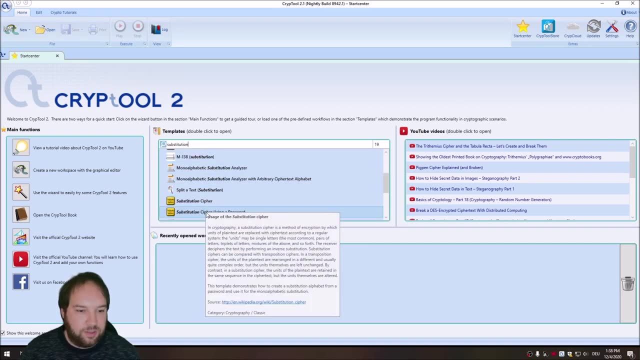 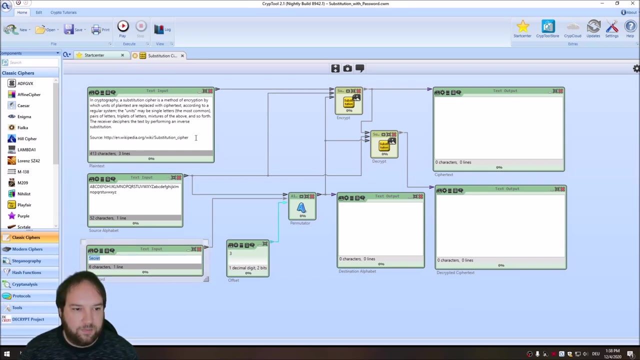 cipher text, and to do so I search for substitution and I take the substitution cipher using a password example. and here we have a substitution cipher with a password. I just remove this here, I encrypt it. we have uppercase and lowercase letters, so I just change it to this here, so we only have the 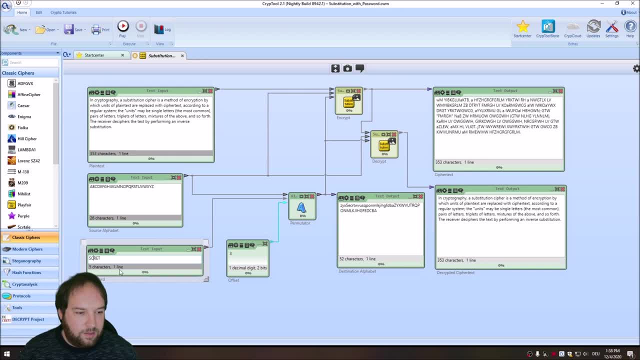 uppercase alphabet. then we have here secret password offset and the permutator here and we also have to change this here to uppercase. now, this was the wrong one. I want to have the string operations with this component. I can change the text to uppercase by just selecting this. 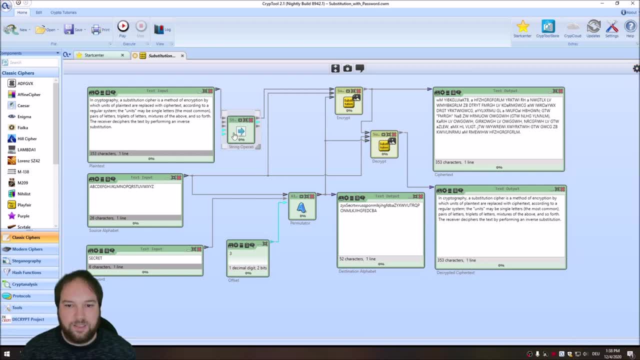 here and changing this to uppercase. so what does this here do? this is, of course, our plain text. the plain text is, with this component change to uppercase letters and with this substitution. here we a component. we encrypt it using a key, and I use here the alphabet permutator to generate a. 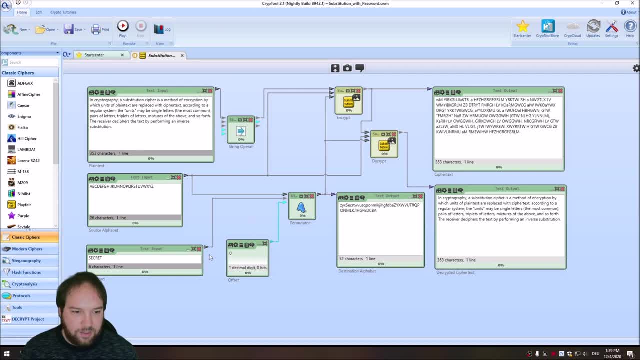 key and I use offset zero, so it will write at the beginning of our encryption alphabet the word secret. of course, with out the second key, we will see the destination alphabet here, and then I want to change the order of the alphabet that is filled after the password for our encryption, or destination alphabet with the. 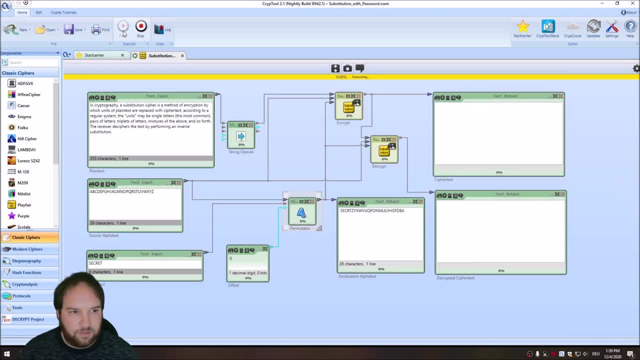 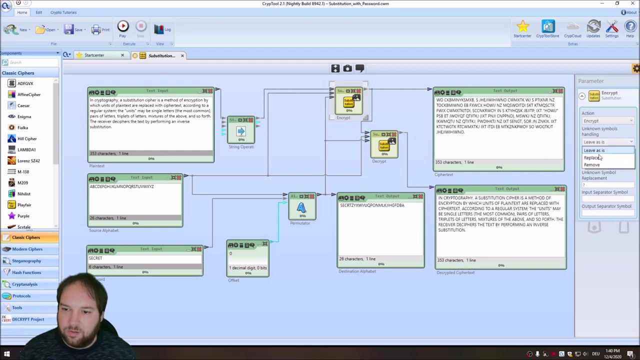 alphabet in descending order, you will see what I mean. just press play and here we have it. we have secret at the beginning of our encryption alphabet and then the remaining alphabet in reversed order. here we have our cipher text and here we have our plain text, and I also want to remove the letters that are unknown. just remove so that we only have 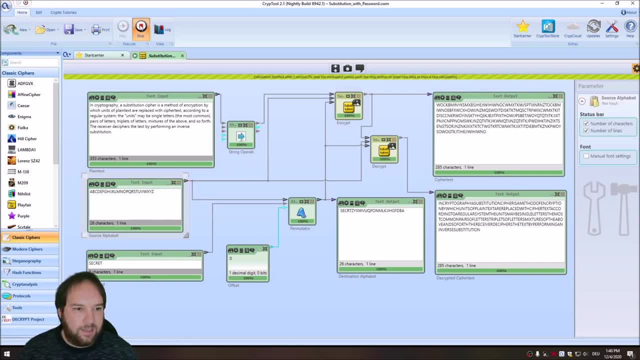 our alphabet letters and at the end I want to have space. so I want to have the spaces. yes, now I have an encrypted text, only uppercase with spaces, so now we can copy this text. it is 340 characters long. and now to evaluate the unicity distance or to have a look what the unity is, the distance helps. 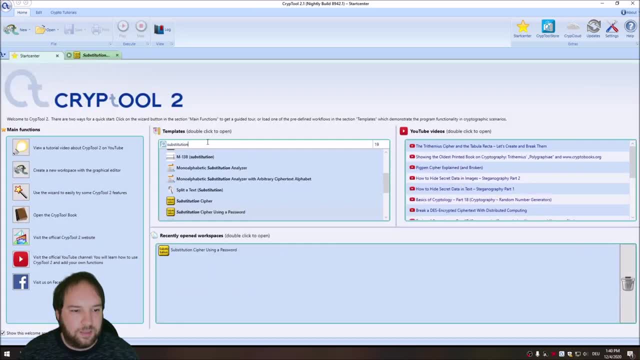 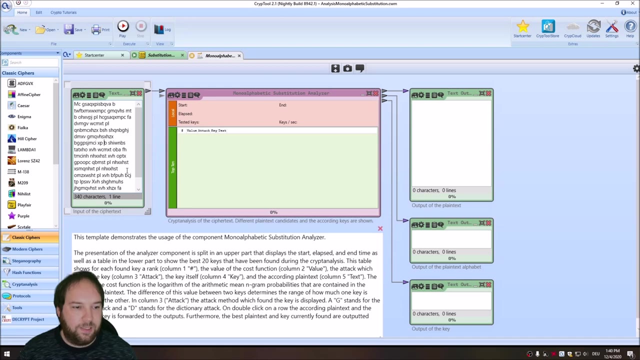 us in decrypting such a cipher text. I want to go to the substitution. oh, it's mono-alphabetic substitution analyzer. where do we have this? here is the mono-alphabetic substitution analyzer and in this template here we can just enter our cipher text. then we have the substitution analyzer. 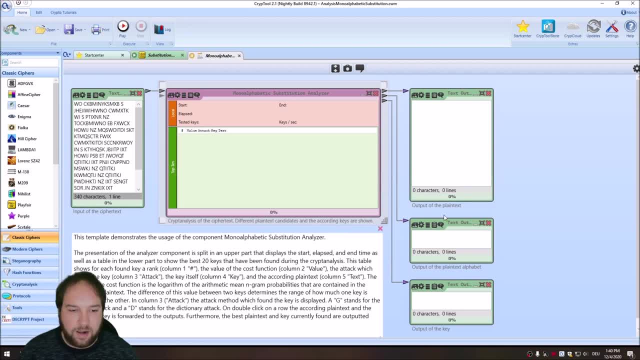 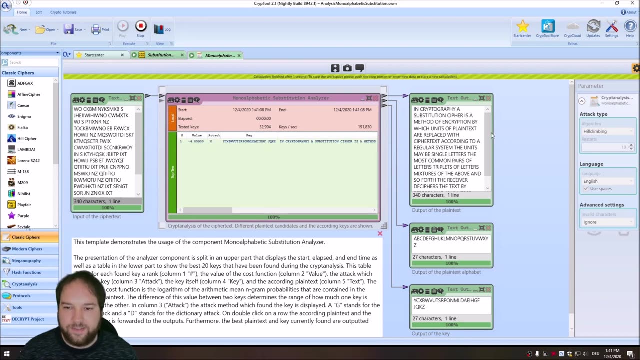 and here we will have the revealed plain text and some alphabets: the plain text alphabet and the key. and now let's test it. we use hill climbing, we have spaces and when I press play- as you know from my other videos, using this component, we can solve this easily. and this is we, because 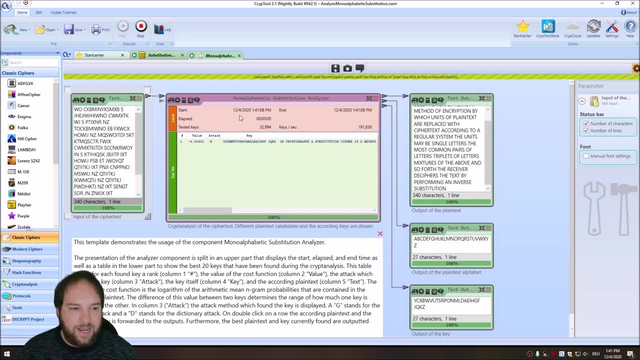 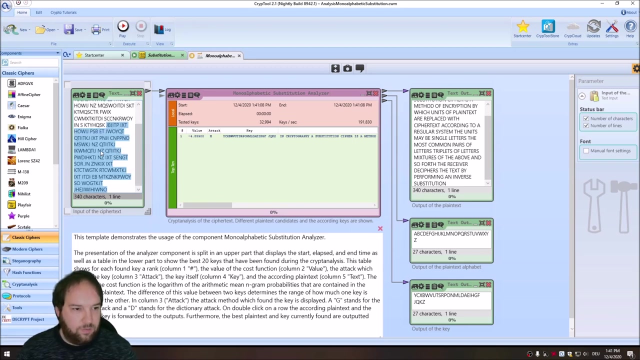 we have a very long cipher text so the analyzer can break very long cipher text very reliably and the text gets the more problems the analyzer has to decrypt or to break the cipher and to reveal the cipher, the plain text. so we will stop this here right now and then no, that was too much I. 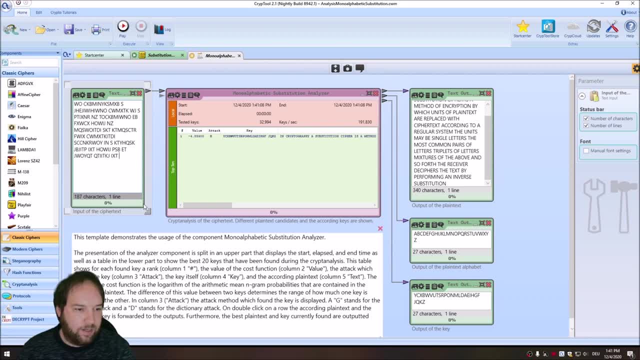 want to half the text to 170 characters. so 170 characters, still a long cipher text. you remember the unicity distance of the simple mono-alphabetic substitution cipher is about 28 letters. so let's play here and we see again in cryptography, a substitution cipher. 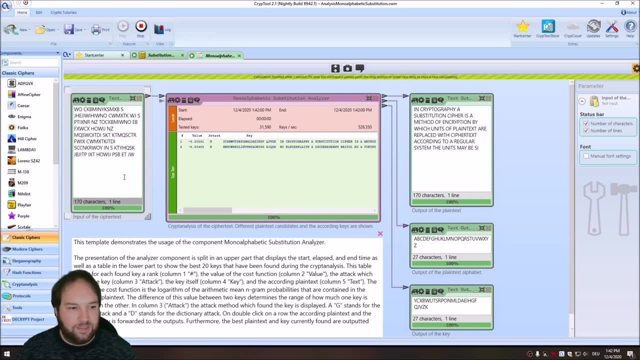 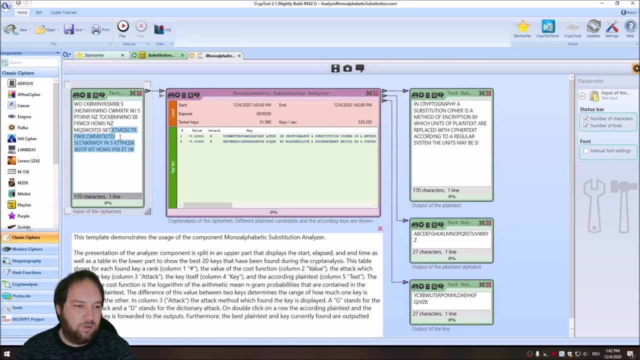 is. it can still solve our cipher, it can still break it, it can reveal the plain text. now we again half the text, so we go to 85 about, or exactly 85 letters here. also keep in mind that it also counts the spaces, so actually it's shorter than 85.. 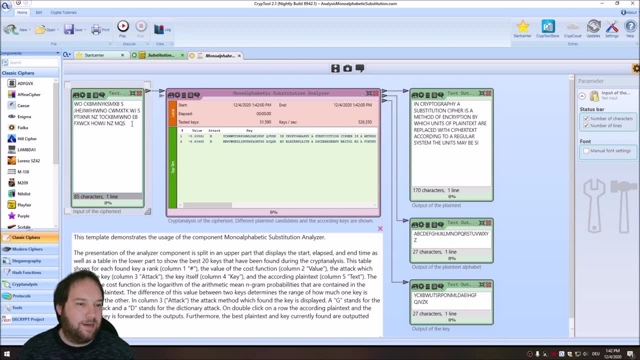 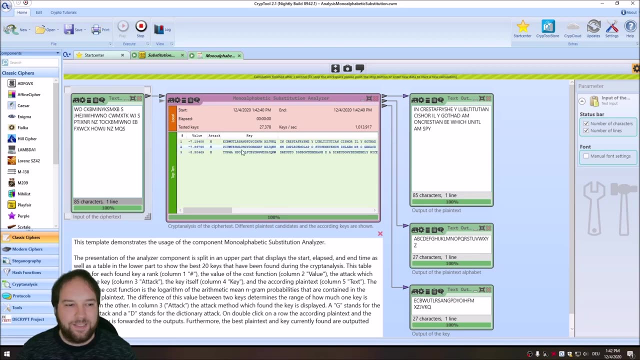 characters. but the spaces in this text are part of the cipher right now because they separate here the letters and that also helps the mono-alphabetic substitution analyzer in finding the correct solution. now let's press play and you see that it starts to get problems here. but this is also based. 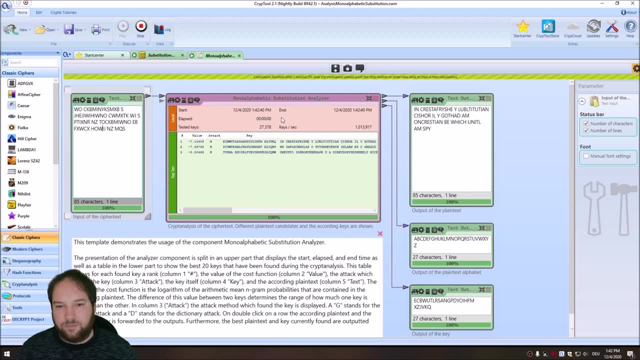 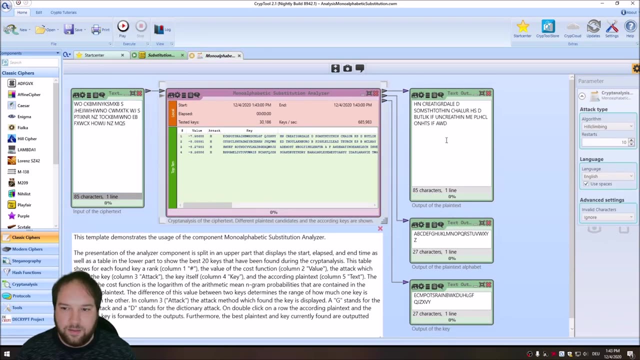 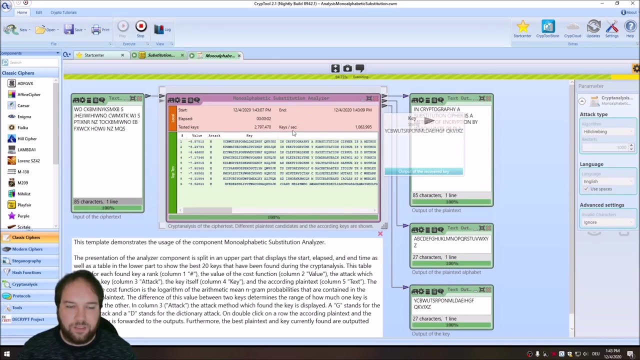 on the fact that the solver is having trouble doing this, that the solver is not perfect, of course, in solving and that's creating such problems, yes, but sometimes when you, when you restart this, so let's go to I don't know- 1000 restarts, then we have enough. so the analyzer of course not always finds the correct solution. 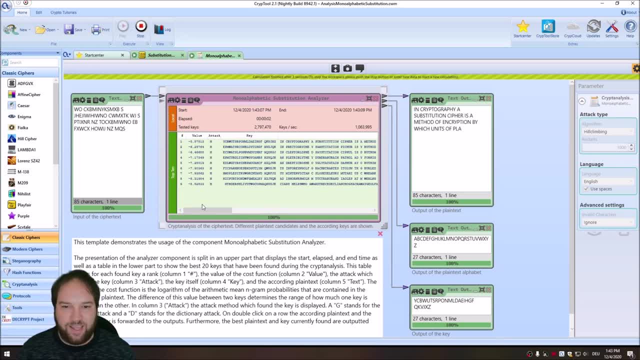 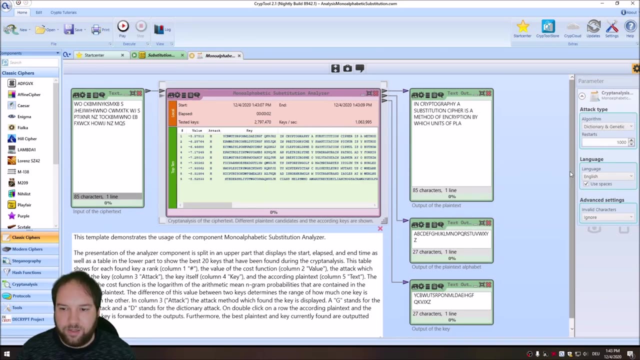 and the shorter the message gets, the more problems the analyzer has. but when you change the restarts of the hill climbing algorithm, that's the crypt analysis algorithm in the background solving this. it also finds this with 85 characters. sometimes it also helps to change here from hill climbing to dictionary and genetic. 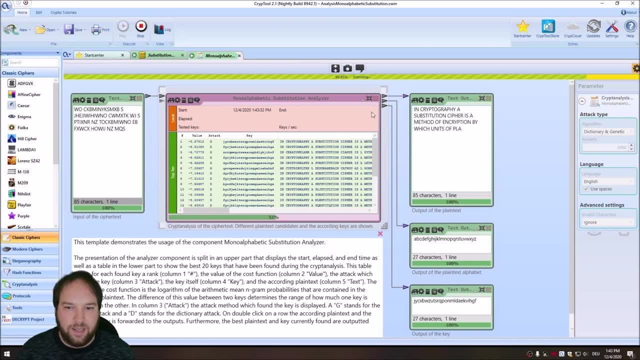 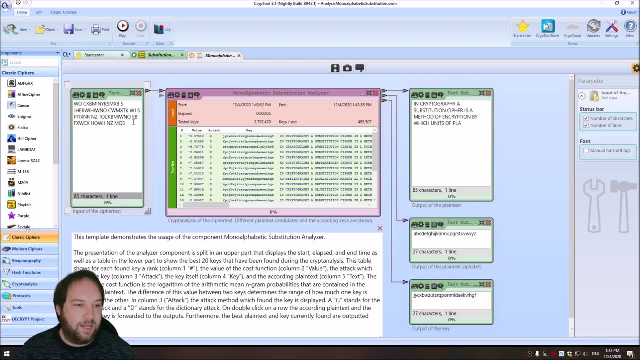 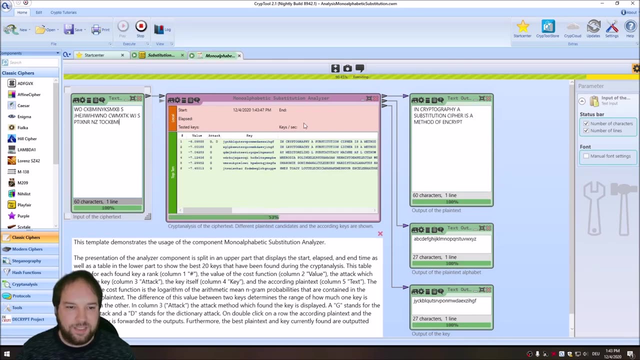 and then, of course, with a genetic dictionary attack it finds the correct solution. I will leave it with dictionary right now, and now we further reduce it. let's go to 60 characters and still with 60 characters. with this attack, with the dictionary attack and genetic attack, it finds. 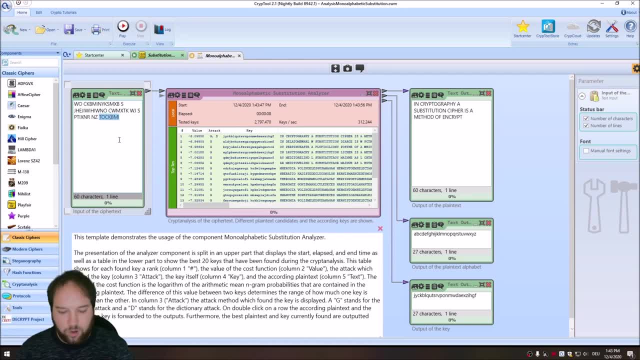 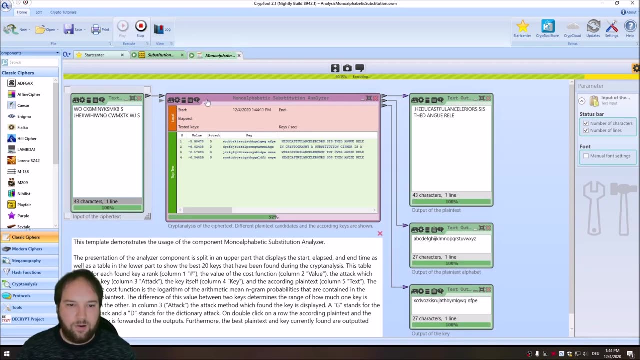 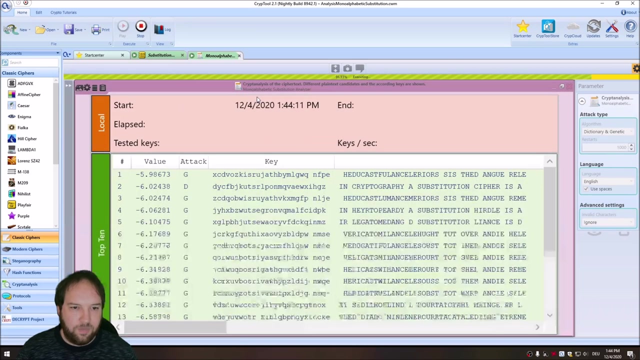 the correct solution. and now I want to remove word by word and test it: still 52 characters and it works. we remove the F, the off, it still works. and now it starts to give us problems because what you can see here, we make this a little bigger. our correct solution is still in our best list here, but using our language model. 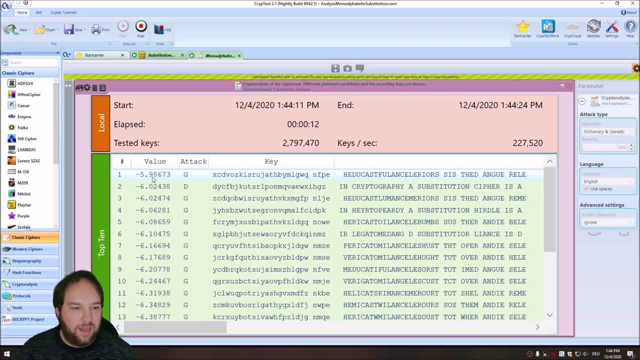 that rates. is this solution English language? we have a better candidate that is above our correct solution. so we have here in cryptography a substitution. cipher is, but it also generated this here where it highly or varied things. this is English, but of course as a human we can see this. 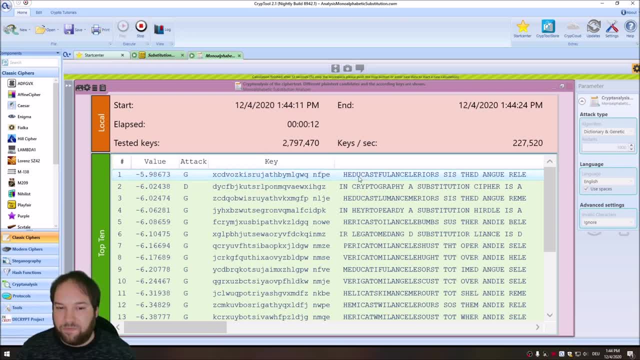 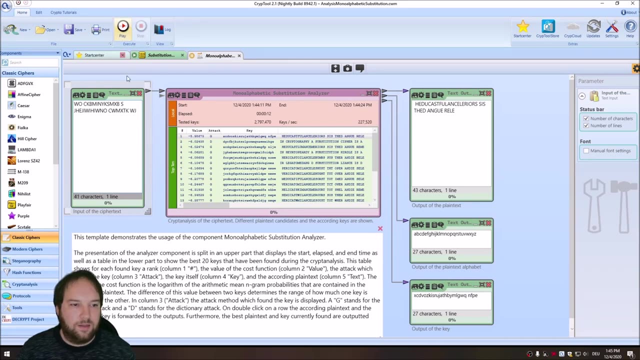 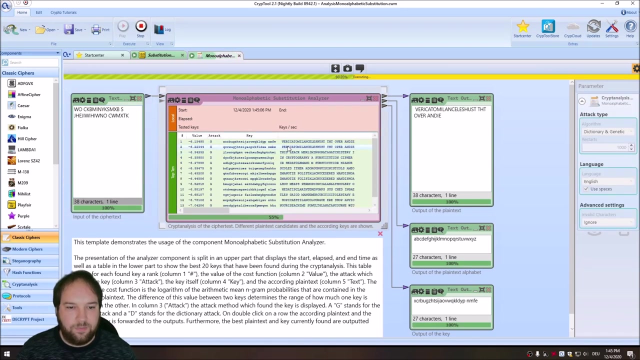 but when you reduce the length, the better the fault solutions will get and also our correct solution will also go below or down this list here and at one point we won't see it anymore. so let's stop this and remove this here. now again, we saw it. but it can also generate solutions that also look correct. here we have. 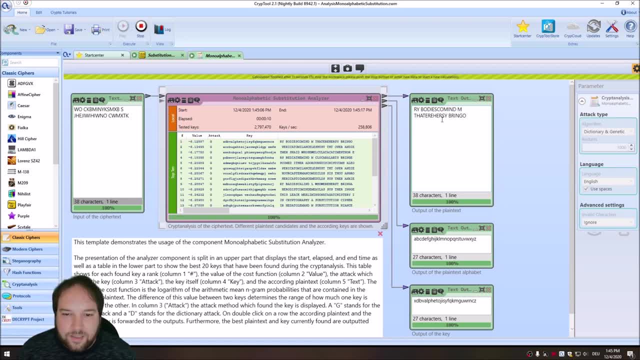 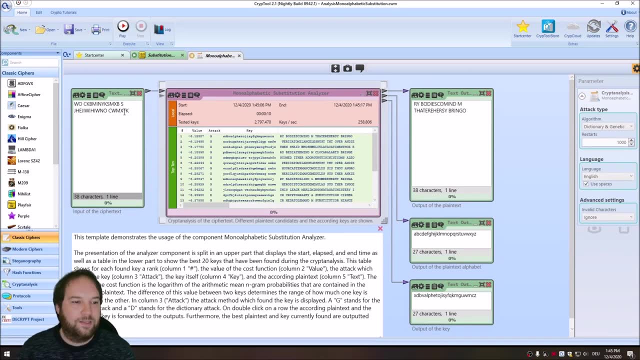 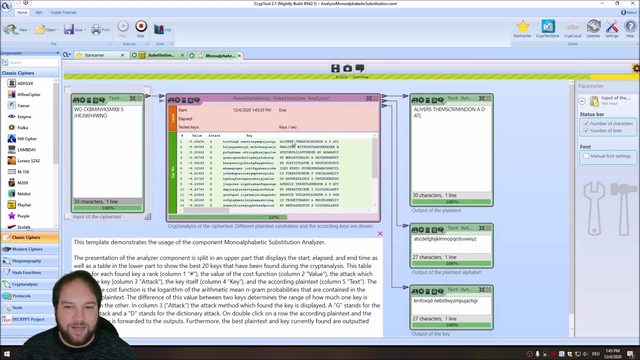 bodies come in Theta. here's a bringo. so the, the analyzer, starts to generate solutions that look like language- let's remove the next one. and also it generates our correct solution. but then it starts also to generate solutions again and again, and our correct solution is now even not anymore. as far as 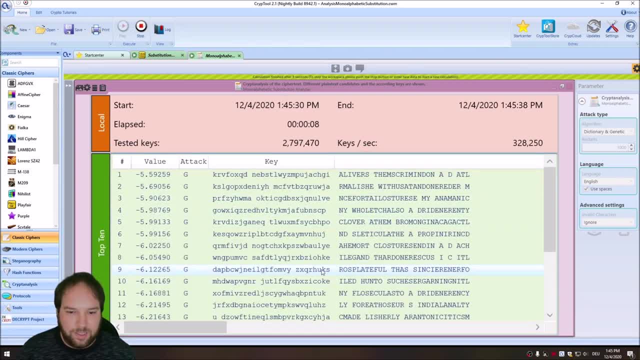 I can see in our best list and you see some parts here look like: here we have a word clover, uh hunt okay, with an O, but here words appear that look like English words and some of these solutions that can be generated by random can actually look like- look like really or real English sentences. so let's remove the next. 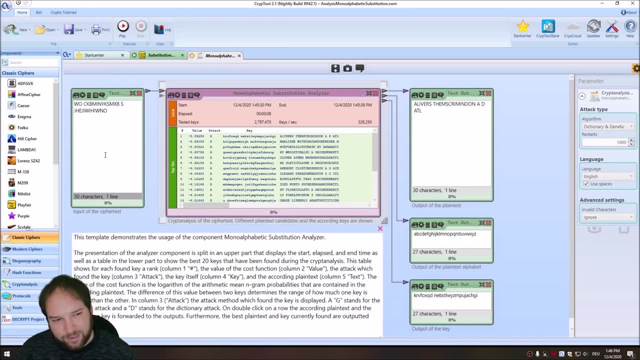 one and with 30 characters we are exactly or really close- not exactly, but really close- to the border of the unicity distance. now let's remove this. we only have 17 characters left. now press play, and I will stop it right now because it generates so many solutions here and we see here, Mothman cares. 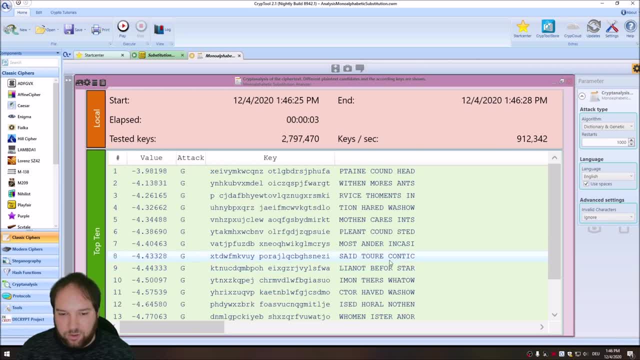 in splint counts that of course there are errors set to a contig, but human is the Anna. so here are some combinations that look like or that come close to real, real English words, and if you would let this run for a while, you will see some sentences that would make 100 percent. 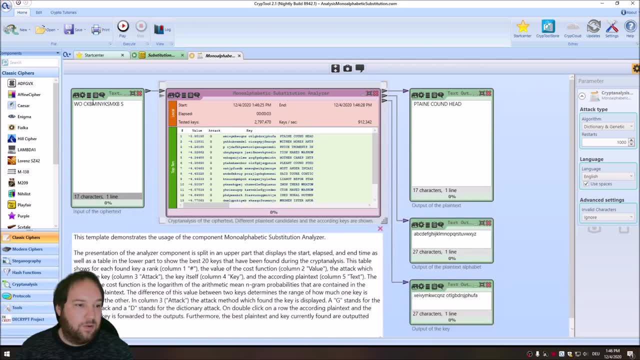 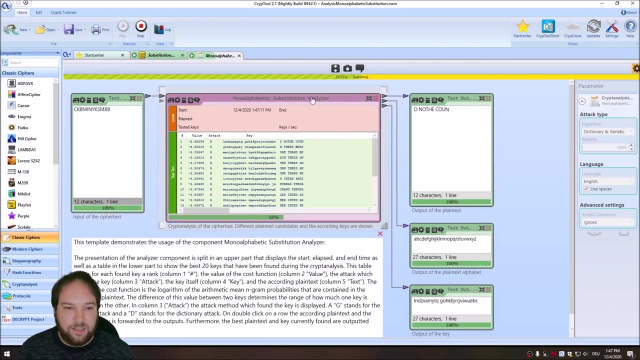 sense to you and when we go even below this. so let's remove that. for instance, that s here and this year, so we have only one word left. I think this was cryptography, I'm not sure. but when you start an analyzer again, also with spaces- you see here one- then B ain't there on, so it. 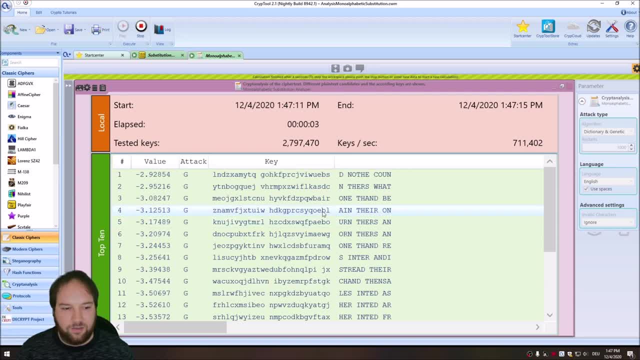 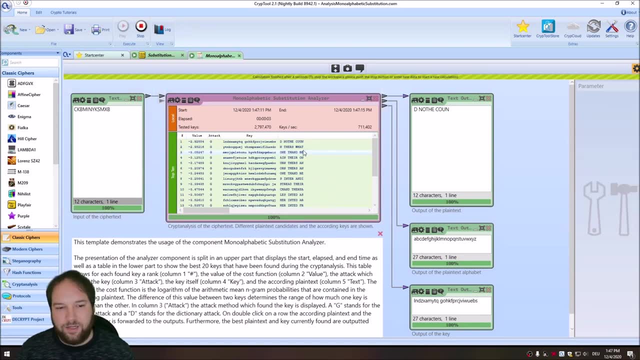 generates things that look like a valid solution. so we are below the unicity distance. right now we have a very substitution cipher and you can generate correct solutions, or our analyzer does this by chance or randomly to generate solutions. so, having a cipher text with a length below the 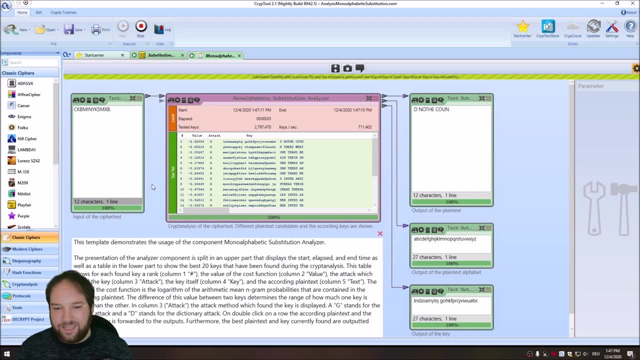 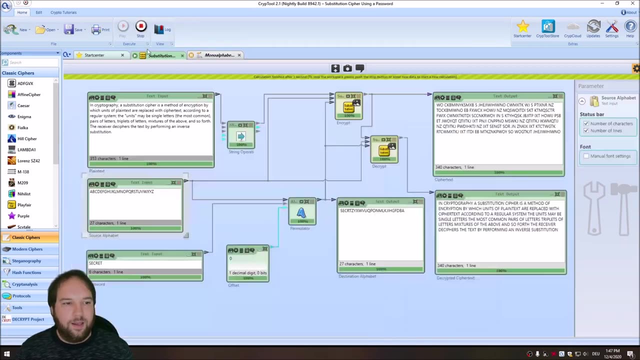 unicity distance of the used cipher. it does not make sense to attack this anymore. you can only decrypt it. actually, when you have the one correct key, then of course you can decrypt it to the correct solution, but you cannot attack it anymore. okay, now let's come to the second part of the practical part of this video here, and this is that. 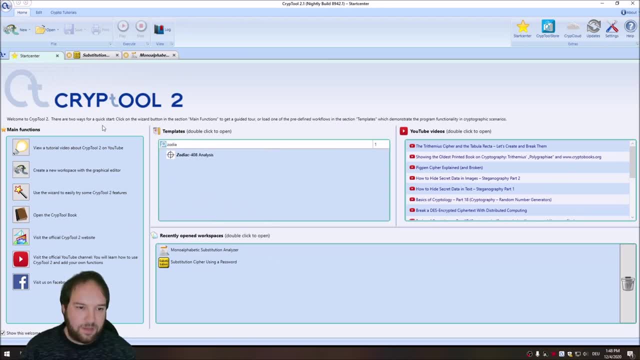 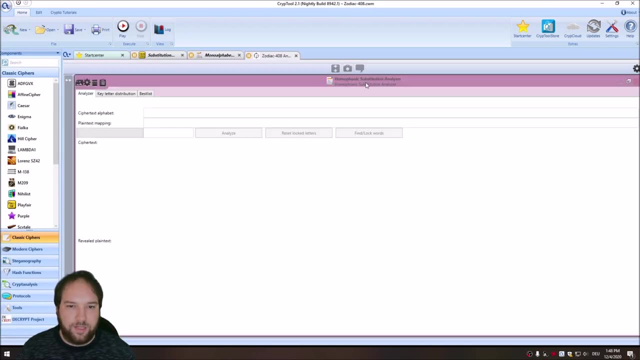 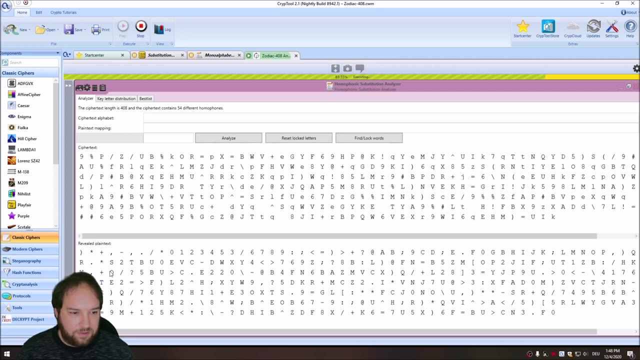 I want to have a look at the Zodiac killer cipher and for that I open the Zodiac 408 analysis and I want to use the homophonic substitution analyzer. so I start it here. here we have the transcription here and here we have the cipher text. here we have the revealed plain text and. 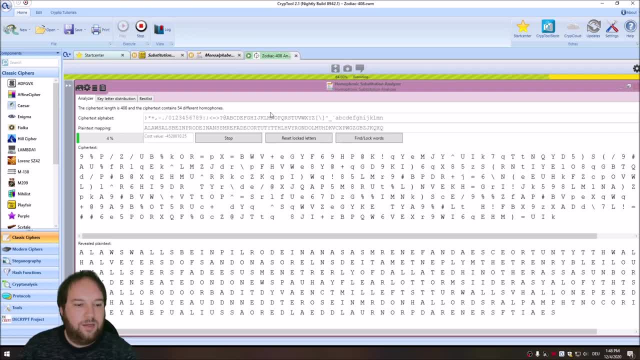 when I start the analysis, it should break the cipher. sometimes we have to restart it several times. it's not so easy to be solved and since this is a random algorithm, sometimes it starts using the wrong start or a false start key and then it runs in the wrong direction. so 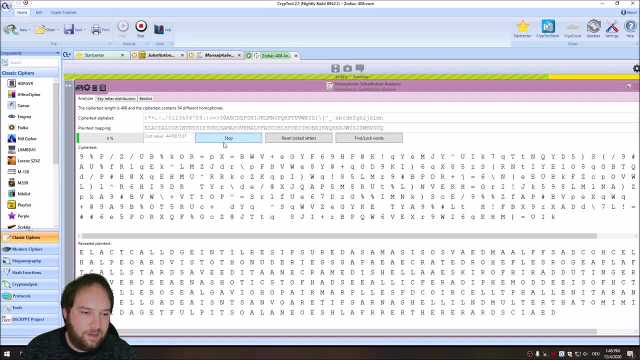 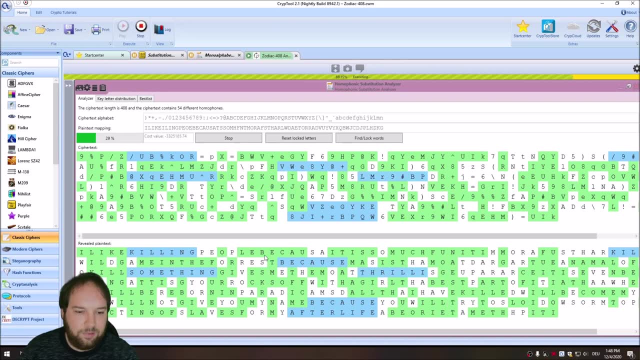 you have to restart it several times so that it automatically- and here we have it because- and then it can automatically solve it. so now let's assume this analyzer would have problems doing this analysis, as you can. as you have seen, sometimes it has problems, but now let's assume that someone gave us only the first sentence. 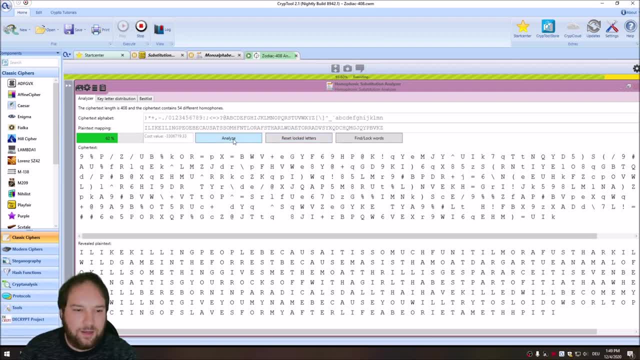 and we want to do this by hand, so I will just start and analyze and then stop so that it shuffles it. so here you see, we have here a random solution and someone told us: I like killing people is the beginning of this letter and, as I said, as an expert I can take the beginning and try to. 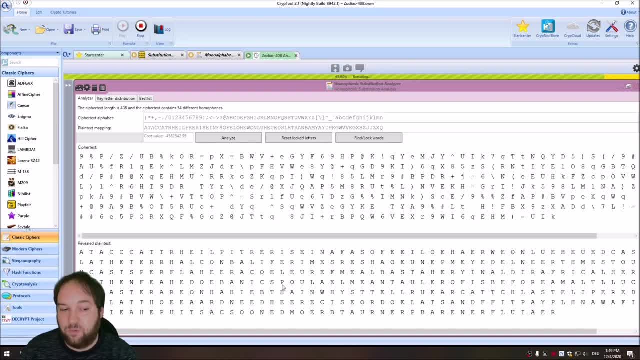 find, with the help of the beginning, if I can solve other parts and if these would make sense. so I just make here I and we have like, and using the homophonic substitution analyzer you can change these by just write, clicking the letters here, and with the left mouse button you can mark these letters here as correct. 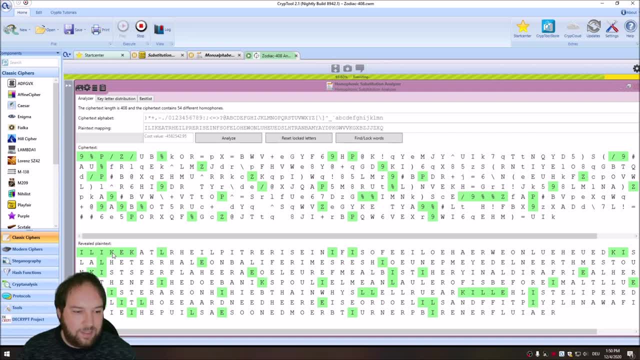 so i assume this is i like and, as you can see here also, this makes sense. the k is used at these two positions. so the solution we got- i like killing- makes sense at this position if we wouldn't have here the same k. we have two possibilities. it could have been an error in the message or the. 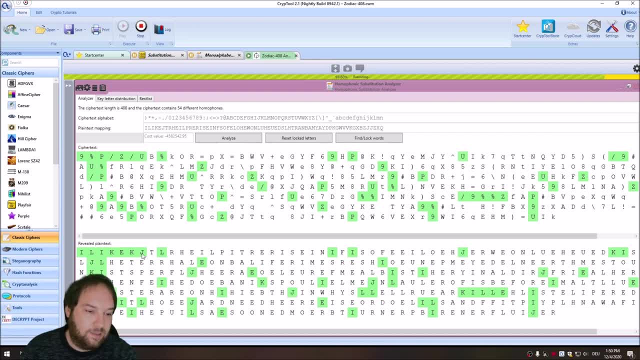 solution is not correct. now we go to killing, so i have i here the l, here kill, and here we have again an l that was used previously. so this also makes sense here to solve it this way, and if you would not have been an l, it could also mean that there's an error or the solution is wrong. now the next is i. 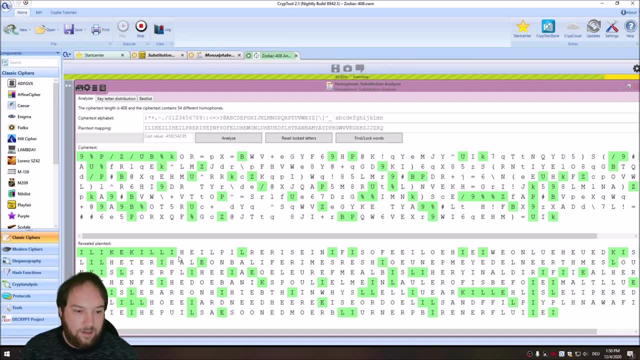 then an And killing G. Now we need people And we also see that this P and this P here makes sense because we want to have people here, And this is the same ciphertext symbol here, So we get P at the same position, So people, so an O and then a second E or a third E. 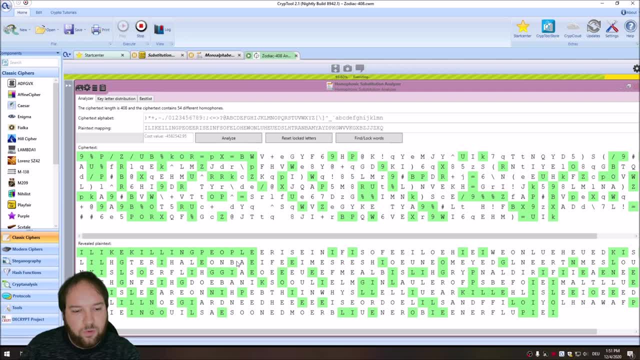 Now we have here. I like killing people And what I would do now with this part of the solution here. I would have a look at the remaining ciphertext and plaintext, of course, and have a look if there are also some part of words or even 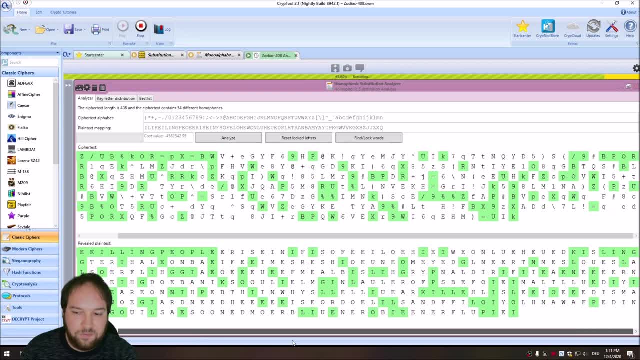 some complete words that makes sense. So, for instance, we see here K-I-L-E-N-G, And of course this would make sense to me to also make this killing. And actually that is what the Hardens did. They thought it could start with. 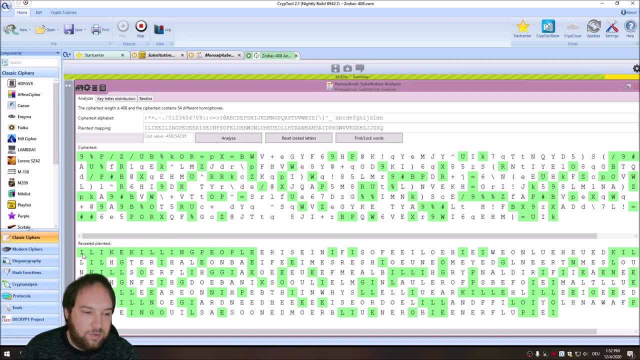 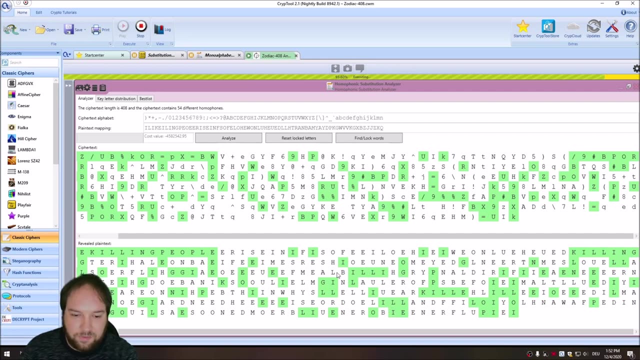 I like killing people this message And using this as a start, they could solve the remaining part, And they also gave this to the expert. that then could also solve the same message. Now we can have a look at the remaining part, So we have a lot of killing here. 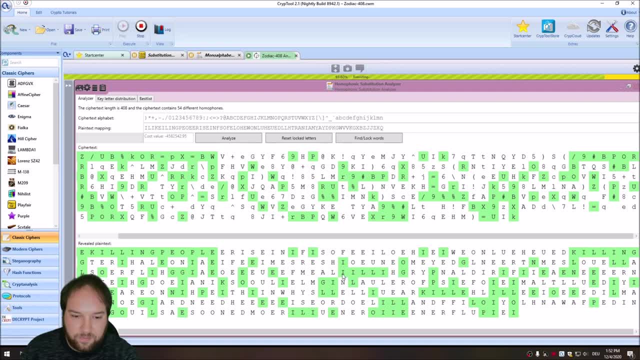 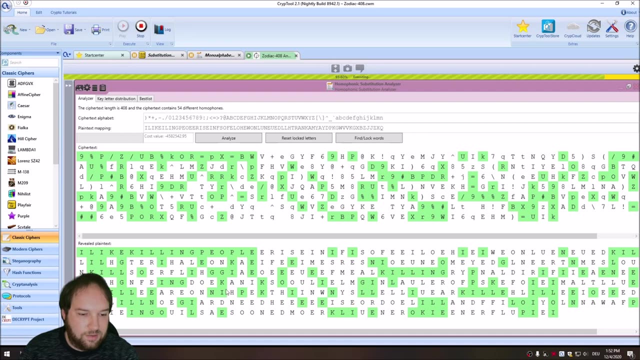 For instance here I would also make this to killing. And then we have here killed, And then what else? Where can we see something? We have a lot of killing, So in this crazy cipher. And then, as an expert, I would go on and try. 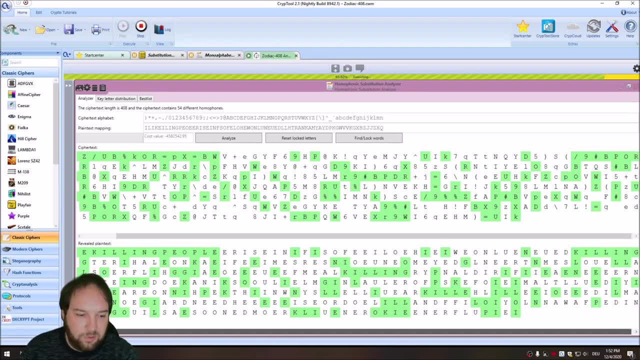 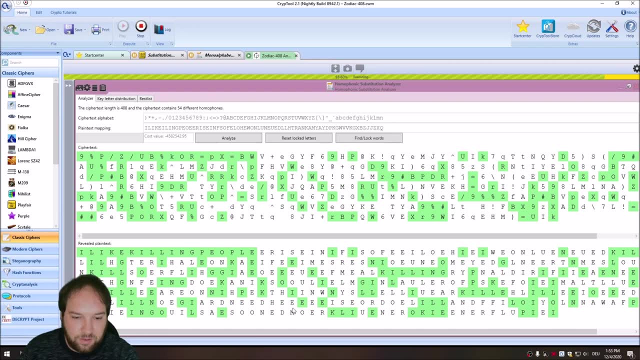 to complete these words here. But of course we have tools today like this one, And when I now click Analyze, the tool can of course go on solving the rest of the cipher using the already solved parts. So I just click Analyze. 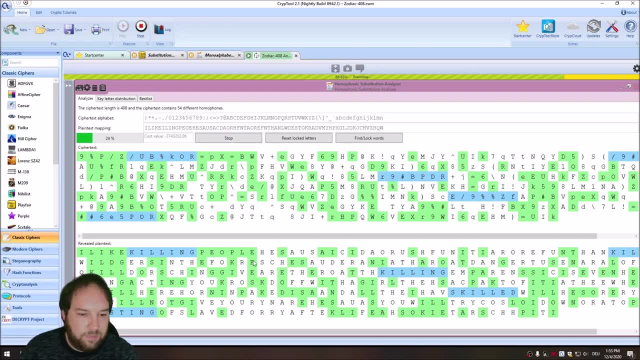 And then we have here- I like killing people. And then, because here's an error in the cipher And using this partial solution, here we have then people, because clearly this cipher text also has some errors. So we have here Because this is E It. 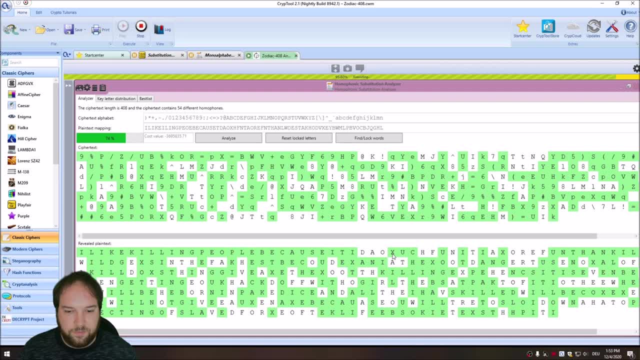 And we have much here And then fun It more fun then. And then we analyze again And so we can reconstruct the original message part-by-part, using The begin that we got and so we can check: is a given solution of a ciphertext is. 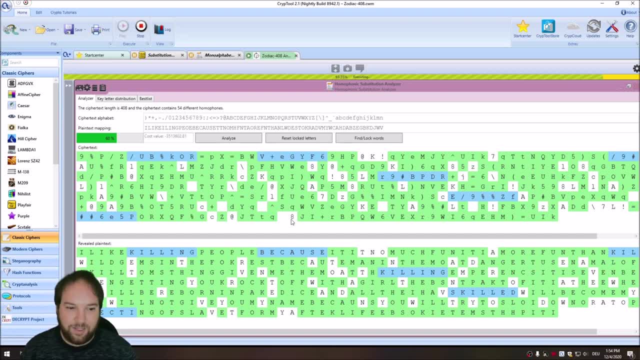 correct. so when you saw it- for instance avoidage manuscript, and you can decrypt easily one page- you can just give this key, how you can solve it, to an expert and then the expert could check if you can decrypt the next page and or decrypt next parts, like from this message here, and when the next parts make sense to. 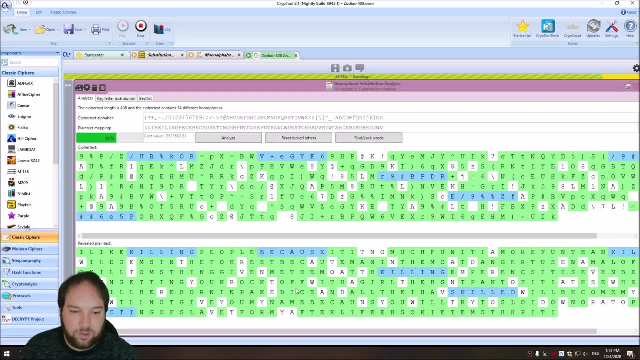 the expert. you can be sure that your solution is correct, and this can also be done using trip to to, for instance, here, as I have shown you right now. yes, and now, when you find a solution, before you contact the experts, use my list: check: is your solution really? could your solution be correct? have a look at the unicity. 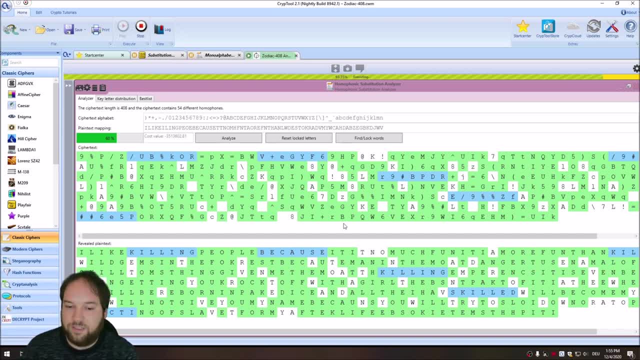 distance of the cipher that you have is that if it's only five letter message, then of course you cannot solve it with a monolith, a substitution and so on, and then you can reach the experts that can help you after that and they also would follow such a list and try to check if your